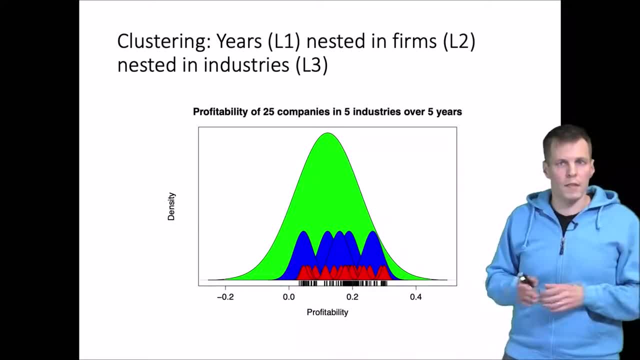 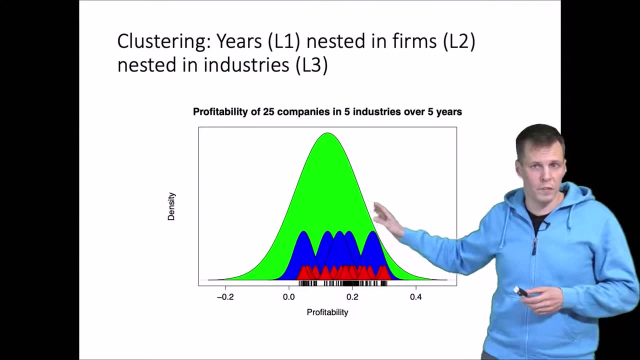 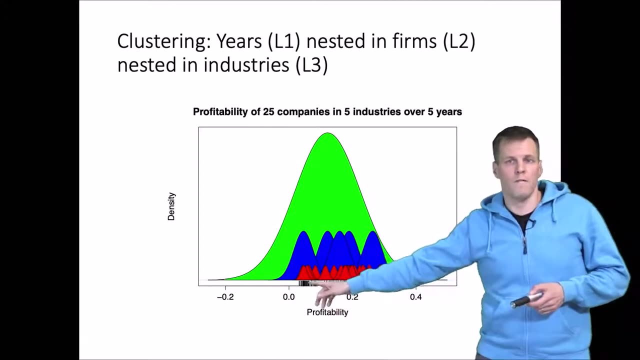 but let's go for an industry level. So we have these blue five different industries and the industries are differing their profitability. Some industries are highly profitable, others are not so And we can see that there are individual variation of the data. here is a function of these. 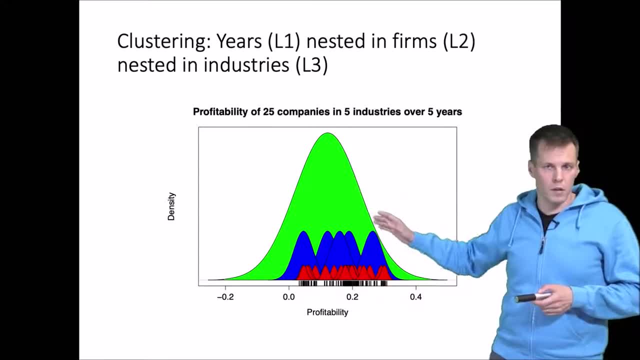 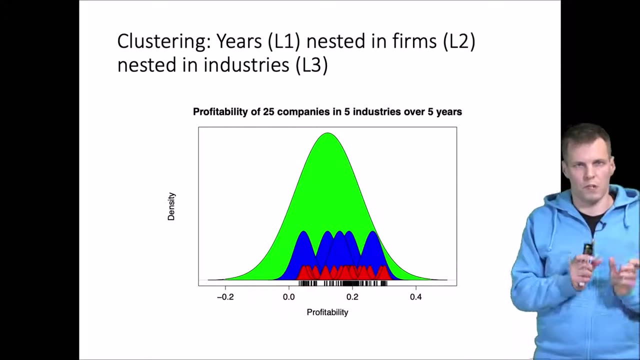 three sources of variation: the between industry level, the between company level and the year-to-year variation within companies. To understand our data and understand the phenomenon that the data represent, we typically need to decompose that variance, to somehow come up with percentages or some other statistics that quantify how much of the variation is here. 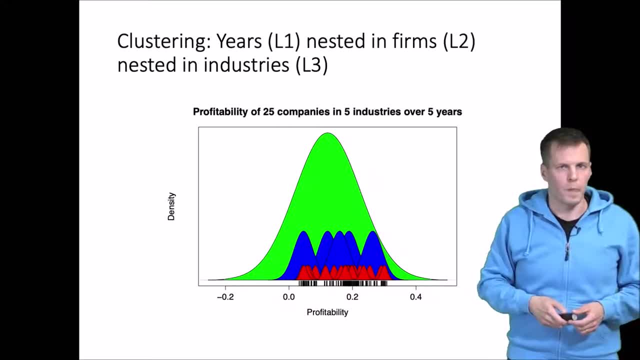 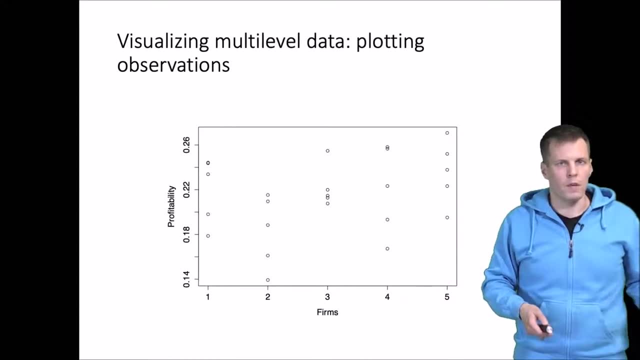 and how much of the variation is here in our data. If our data set is small, we typically start with a graphical analysis, So we can just plot the data. This is 25 observations, five observations for each company, for five companies within one industry. We can see that. 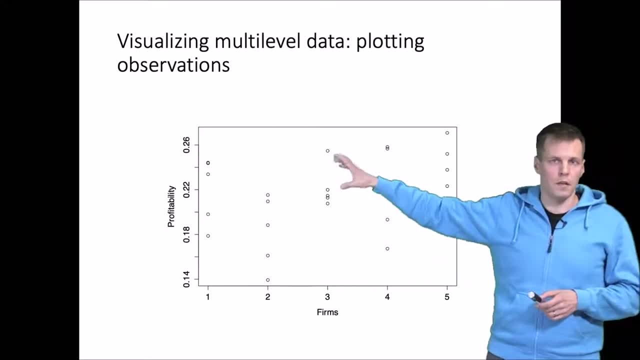 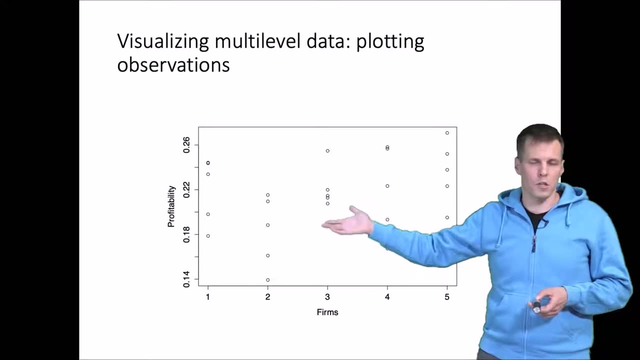 there are some patterns. For example, this company, there is not much variation in performance, This company is less profitable than that company, and so on. This kind of analysis works well when you have a small set of observations. If we have a large number of observations, 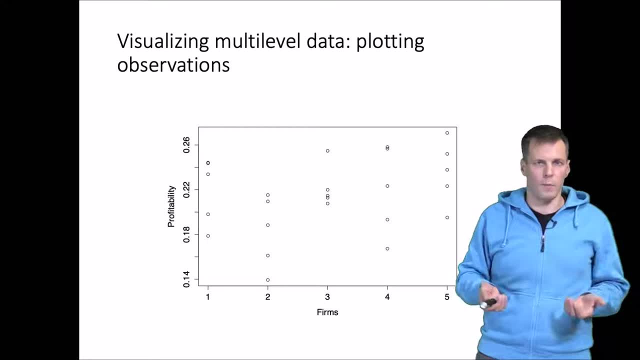 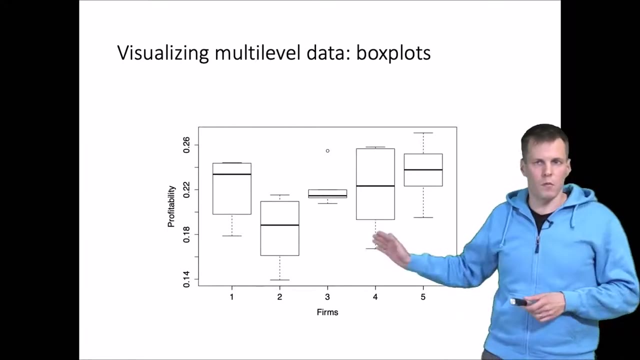 but still a fairly manageable number of clusters, let's say up to 30 companies or 30 industries or whatever is our level two unit. we can use box plots. Box plots are graphical representations of variation of individual variables and we can do box plots by groups. The idea of a box plot is: 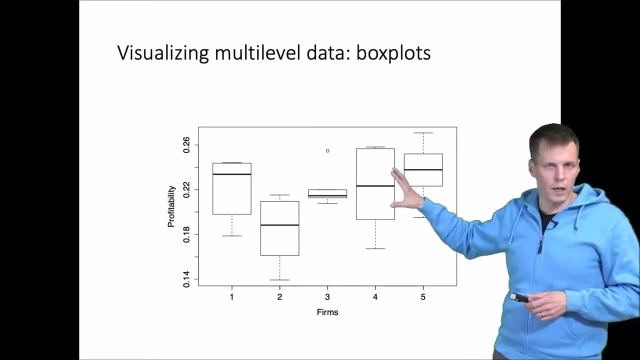 that we first calculate for a variable. we calculate the median and the median gets this thick line here That marks the median. Then we calculate the first quartile and the third quartile of the data. So quartile means that below this line lies 25 percent of our observations and above the line 75. 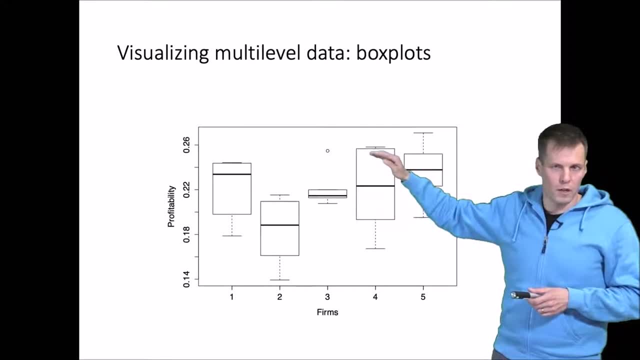 percent. median is half and half and third quartile is 75 percent and 25 percent. We draw a box between the first quartile and the third quartile and half of our data is within this box. Then we have this whiskers that indicate the minimum and maximum and sometimes we also have outliers that the box 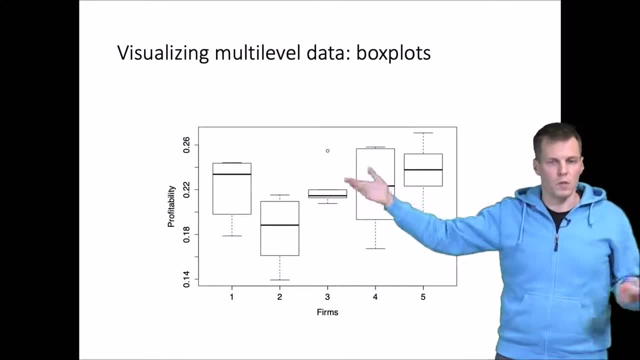 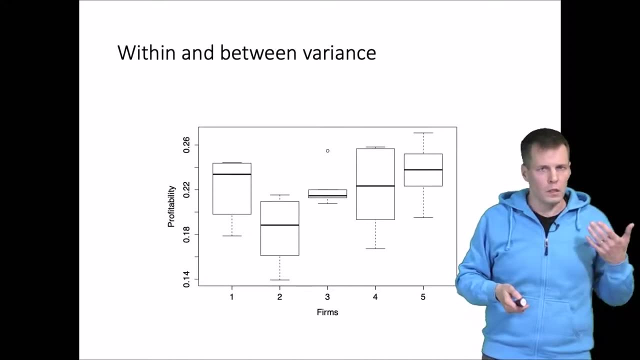 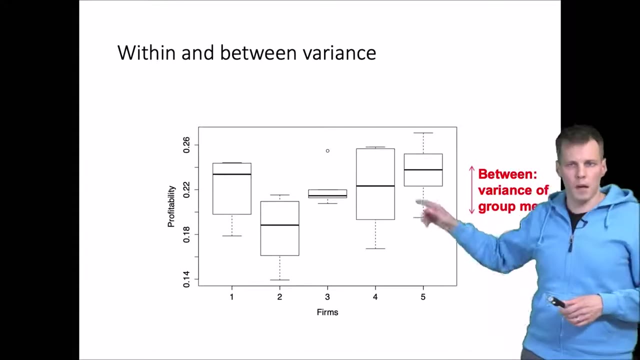 plot algorithm identifies as circles. So why is this box plot presentation useful and how can we analyze the box plots? We can first of all start to understand the between and within variance by looking at the box plots. We can compare these medians, or we can do box plot with means and we 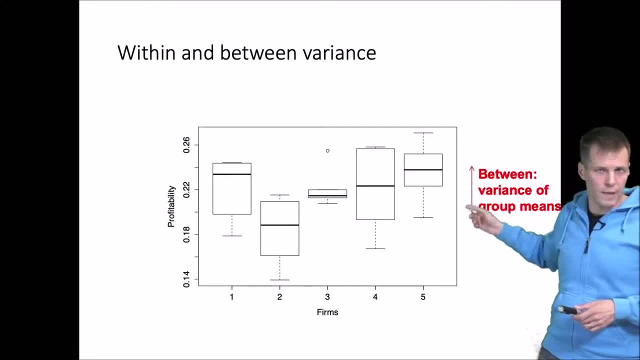 can also use the box plot method. So what we can see here is that if we have a box plot with means, then we can use the box plot method to find out how much variation there is between these means or medians, and that is our, our between variation. We can also take a look at how high the boxes are. 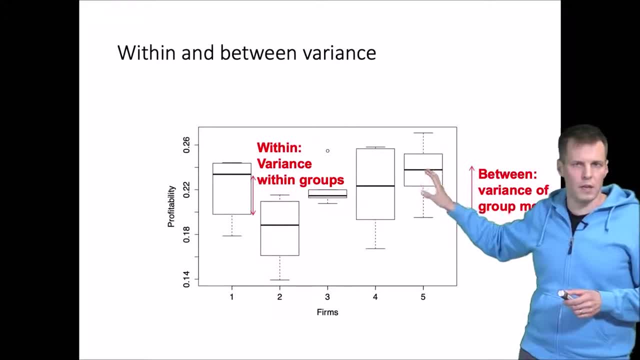 and that quantifies the within variance. Comparing these two studies, these two dimensions, tell us if the variation in this variable is more due to the differences between firms or is it just random. is it a within firm or between variation? that explains the data. We can quantify the level of. 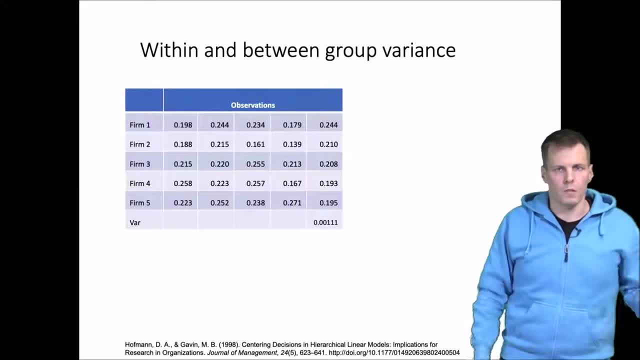 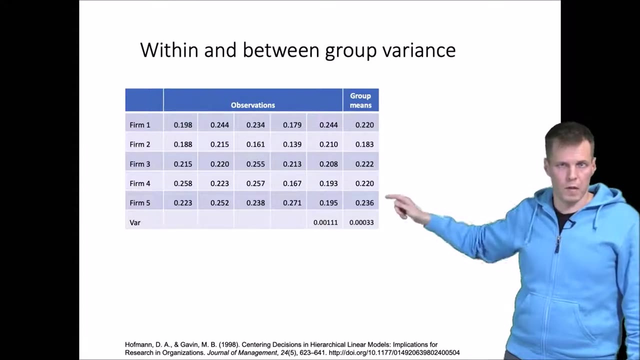 variation between two levels, also numerically, by calculating the within variance and between variance. This is our data and we start by calculating our group means. So we take each of these companies and we calculate the mean of this. So that are, these are the group means, or? 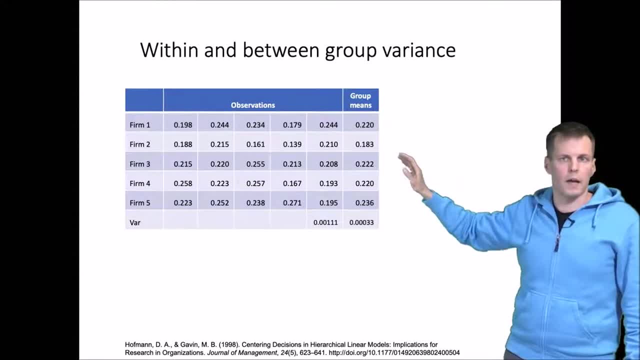 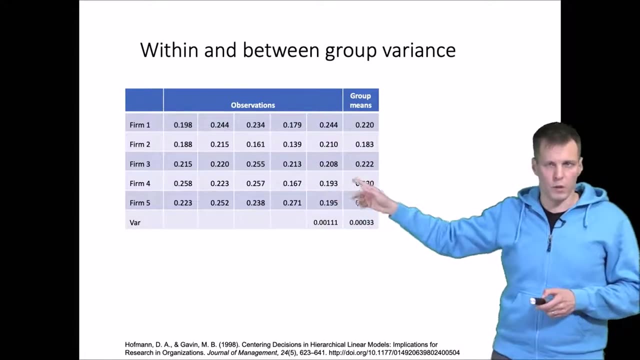 cluster means for these, these five firms, and we check how much these means vary. The variation is quantified here with this statistic and then we calculate how much these individual observations vary from the group mean. In practice we do group mean centering, so we take each of these observations. 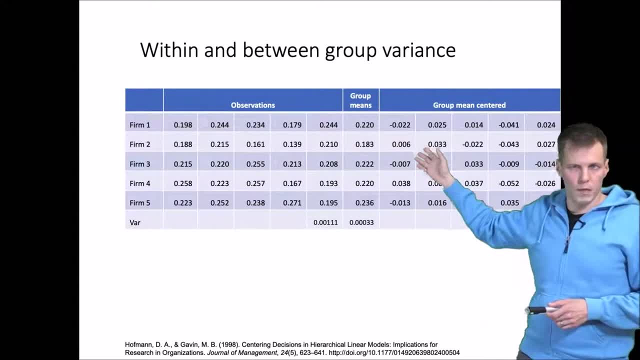 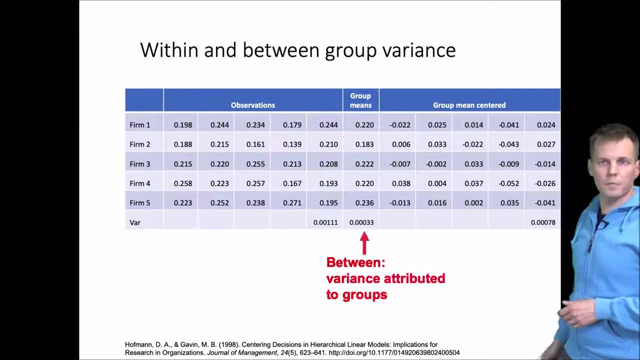 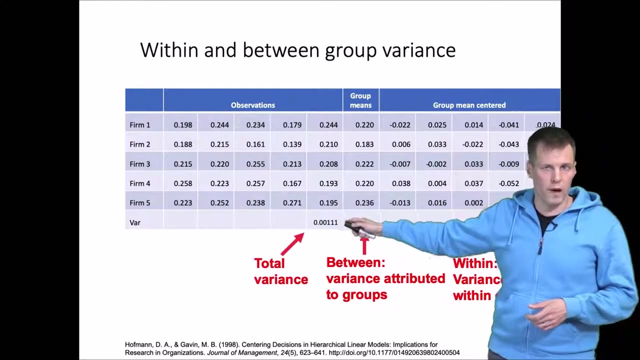 we subtract the group mean and that gives us the group mean centric values. Then we calculate how much the group mean center data varies and this is our between variation, this is our within variation and this is our total variation, which is the sum of the between variation and the within. 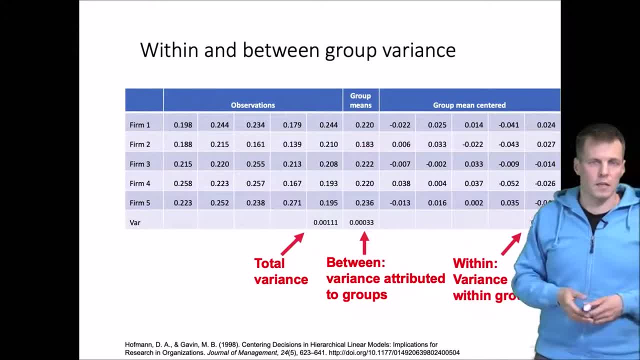 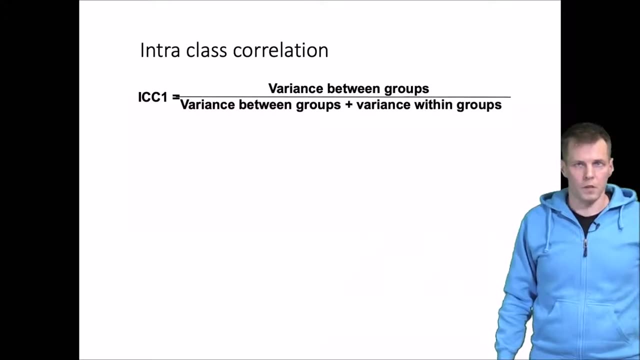 variance. So the variation or variance is a statistic that depends on the scale. It would be useful to have a scale free way to explain on which level the data varies, and this is where the integral class correlation comes to play. So integral class correlation is simply: 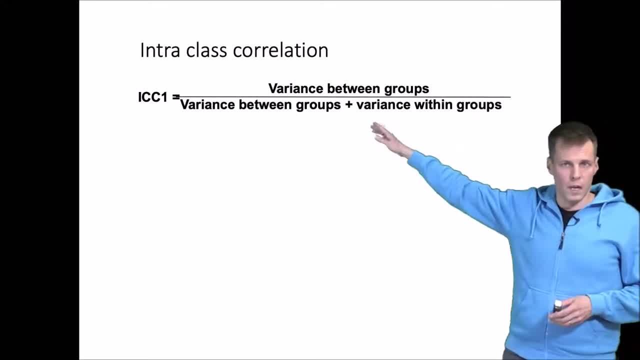 calculated as variance between groups divided by the total variance. So it answers the question how much of the variation in the data is attributed to the groups and how much is attributed to the variation within the groups. This is called ICC1 for reason that there are 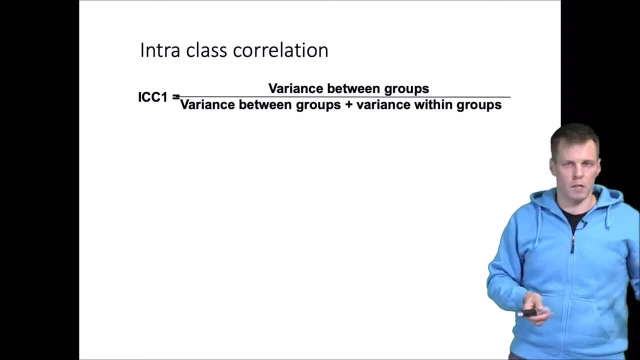 many other kinds of integral class correlations. So integral class correlation generally refers to a correlation between observations and, because there are many, this is called the ICC1.. There are like a few others, but this is the most important one that you need to understand when you work with multi-level data. Other integral class correlations. 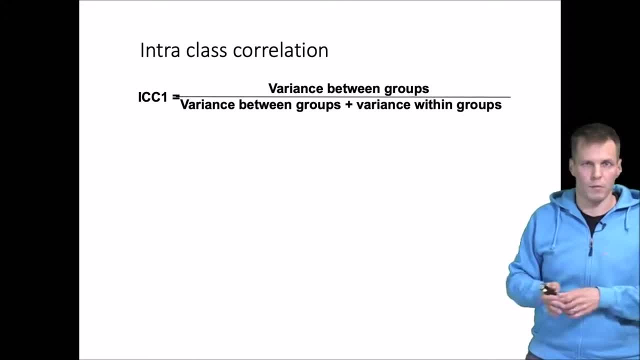 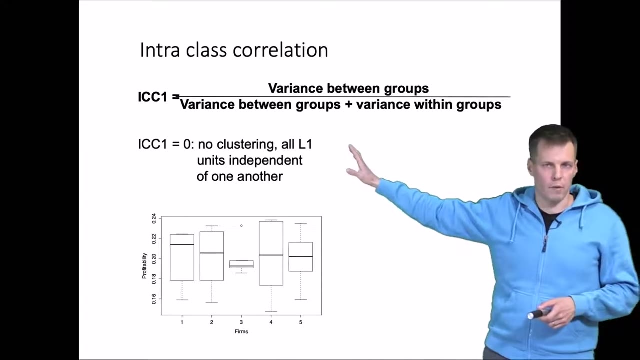 are mostly about reliability of multiple raters. but ICC1 is this simple equation that simply quantifies various. When ICC1 is 0, then that indicates that there is no variance between groups. So the box plots are all on the same level. here there are no difference. 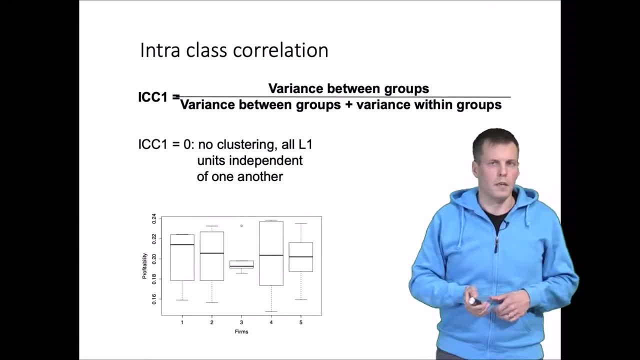 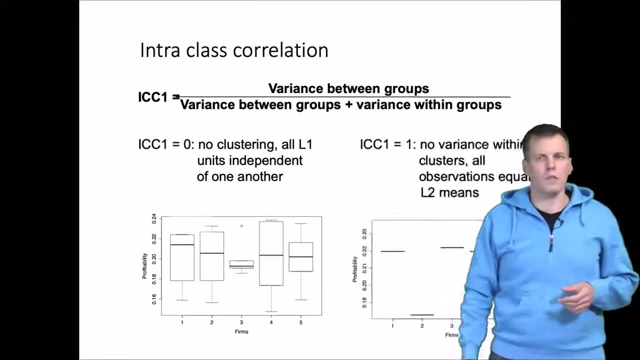 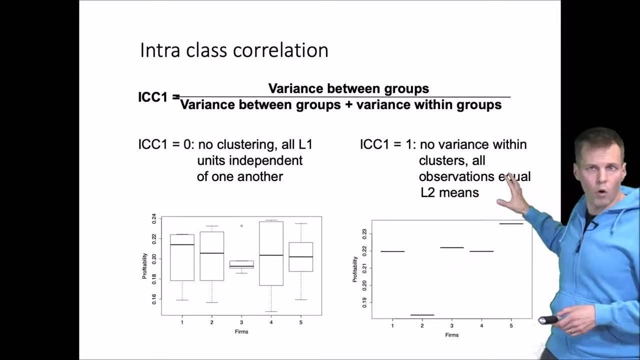 between means, and in this case medians are close as well, and all variation is simply because there is variation within these groups. Then when intraclass correlation is one, then that means that there is no variance within clusters at all. all observations equal. the level two means So: 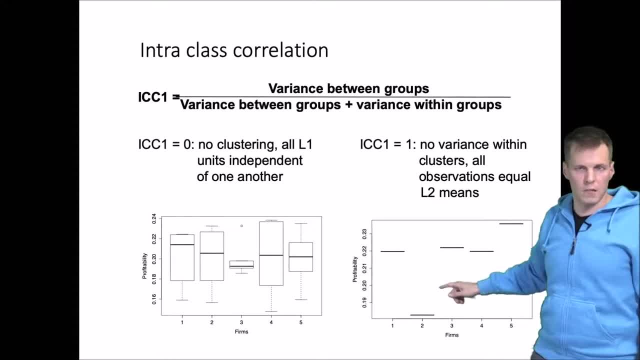 this firm's profitability is always here, this firm's always here, and so on. So there is no within unit variation. Why do people calculate intraclass correlation and how it's typically reported? The role of intraclass correlation: the first role is to make a decision whether 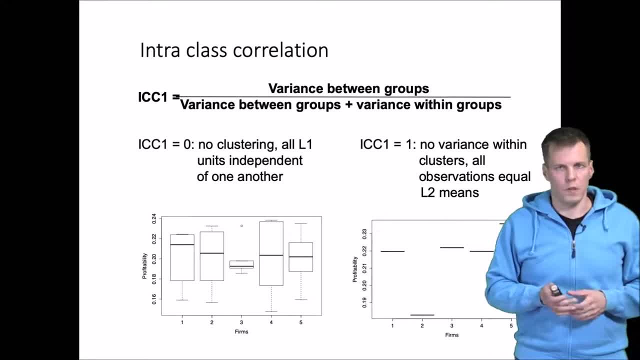 something needs to be done for the cluster. If all the observations within cluster are the same, then you can just pick one observation for each cluster and use those in regression analysis and it doesn't really matter that you have the remaining observations because they don't provide you any more data If ICC1 is zero. 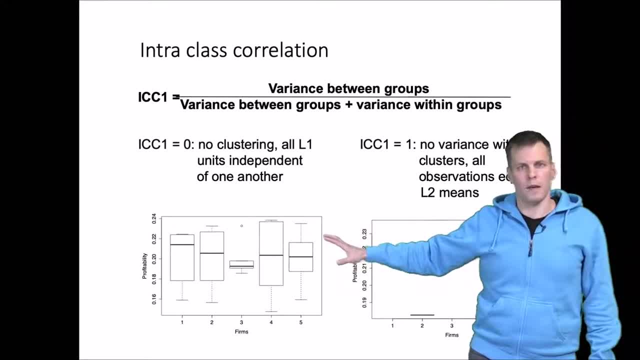 then there is no clustering in that variable. and if all your ICC1s are very low, then there is no meaningful clustering effect in your data and it's possibly safe to go without a multilevel modeling. There are exceptions to that rule, but generally when ICC1 is.